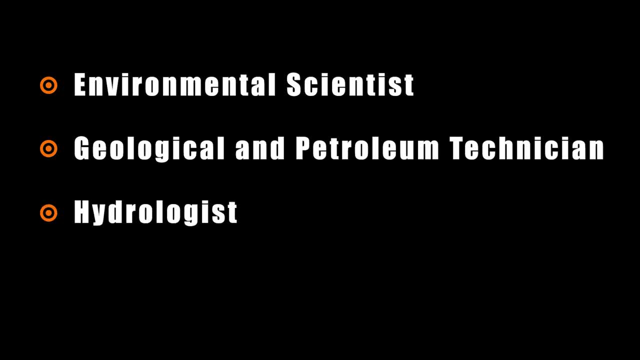 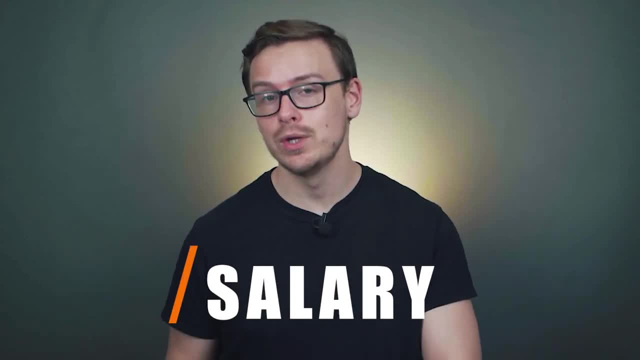 Natural scientist: geological and petroleum technician, hydrologist and natural science manager. Now, the first section we're going to go over- because this is a personal finance channel- is going to be the salary or earnings potential. Now you might become a geoscientist, for instance. 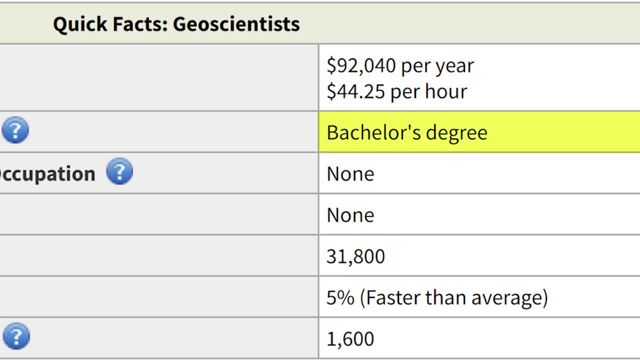 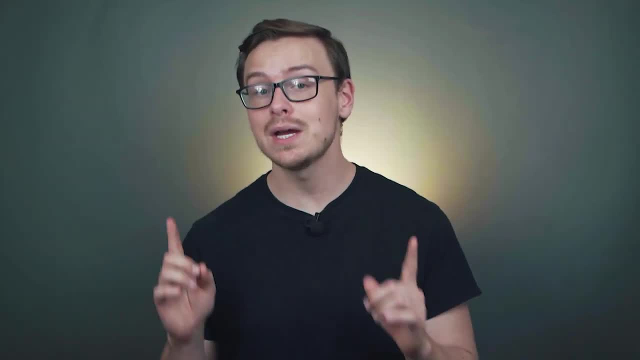 and they make around $92,000 a year with just a bachelor's degree. And when it comes to careers, you might be surprised to learn that you tend to make a lot more later on in your career, and that's especially true when it comes to geology degrees. So, for instance, when you're in your late career you'll be making almost twice as much as what you were making when you first started With a geology degree. you can expect to make around $48,000 a year starting out and $89,000 in mid-career pay. Compare this to a very high-earning degree like petroleum. 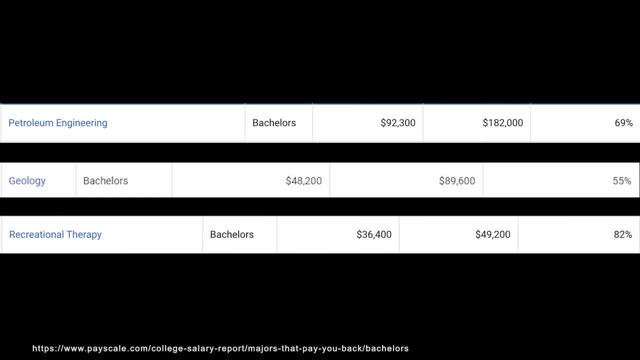 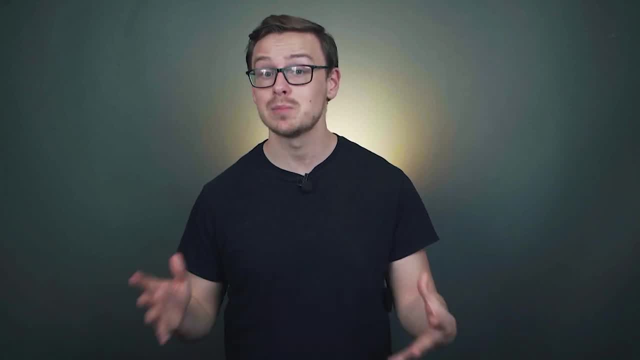 engineering or a low-earning one like recreational therapy, and you'll see there that it's on the higher side, definitely above average. So this one's above average, especially for a science degree, but it's nothing special compared to all other degrees, So I'm going to go ahead and give. 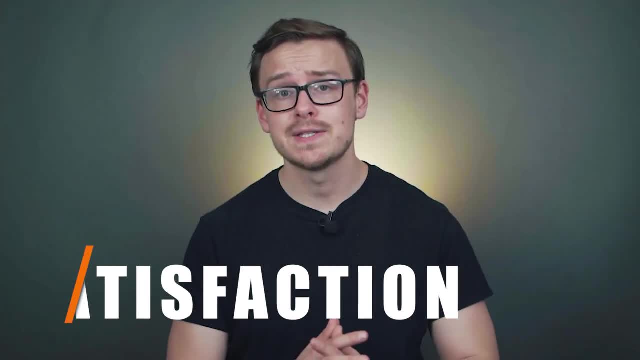 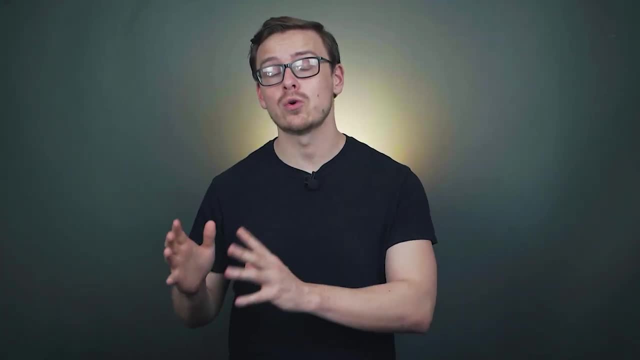 this one, a 7 out of 10 for salary. Next, we're going to talk about satisfaction, and I usually talk about job satisfaction and meaning. So when it comes to meaning, that is how much you think your career positively impacts the world. So you might hate your job, but at the end of the day, you know that you're. 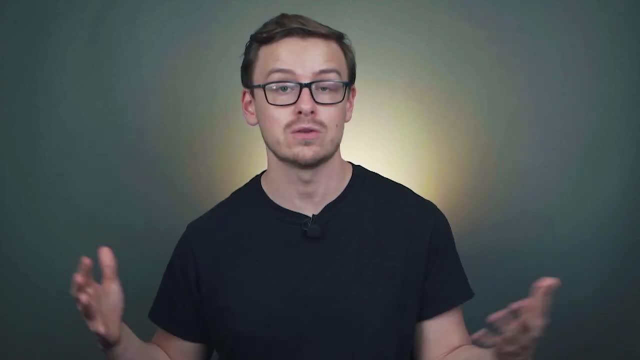 really helping people, and so you know that it's positively impacting the rest of the world, which is a good thing, Whereas job satisfaction is just how much you enjoy doing your job. Depending on the person, one of them might be more important than the other. Now, overall, 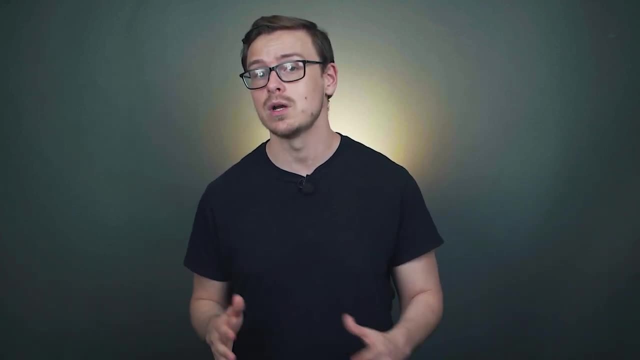 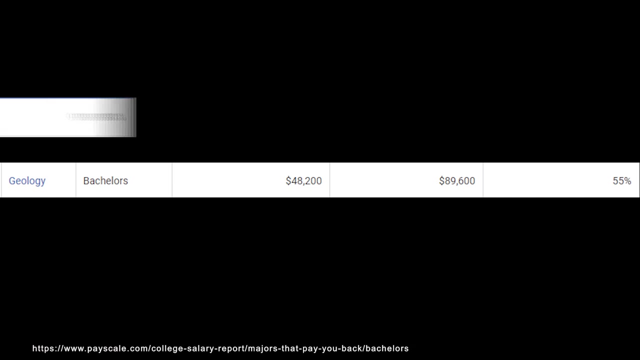 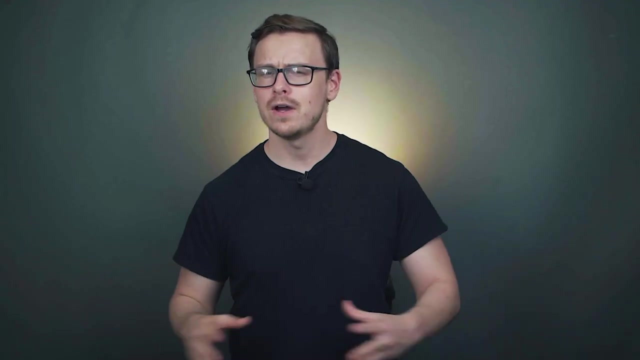 satisfaction is extremely subjective, but I try to be as fair as I can when I'm talking about these. A biology degree is going to have a 55% meaning score, with a high meaning score being radiation therapy at 91% and a low meaning score being plastics engineering technology at 31.. 55% is 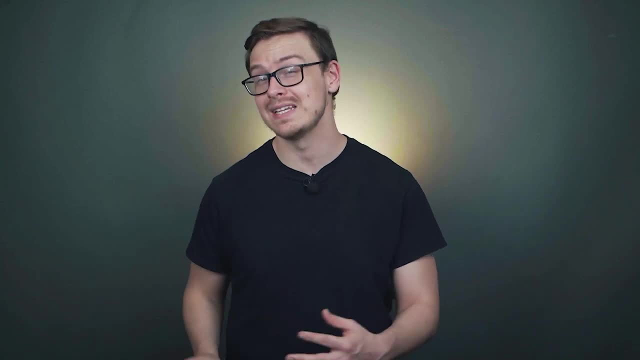 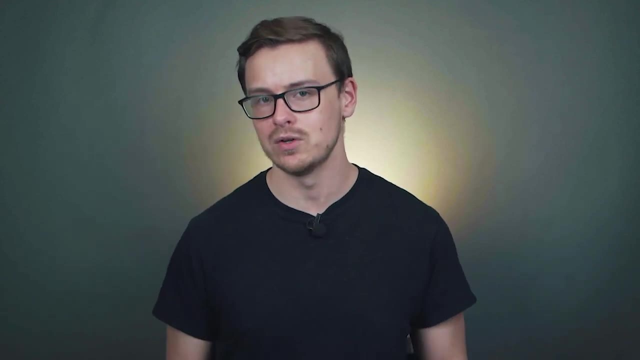 slightly above average. I would say that's about average for a science-related degree. Science degrees tend to have higher than average meaning scores, and so I'd say that one's about average or slightly above average. And when it comes to job satisfaction, you see that geoscientists have. 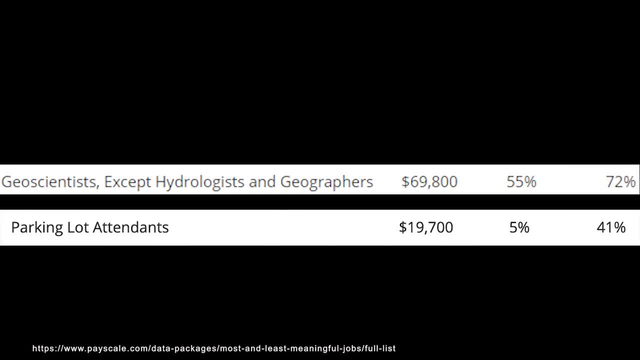 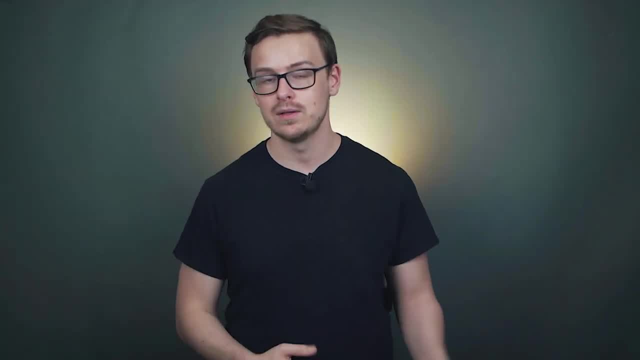 about a 72% job satisfaction score. Again, a low score would be 41% and a high score would be 90%, and so 72% is above average as well. And, like I said before, people who get a science degree and then they're able to actually get a 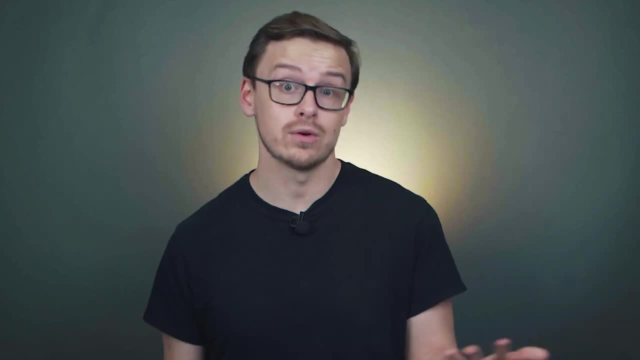 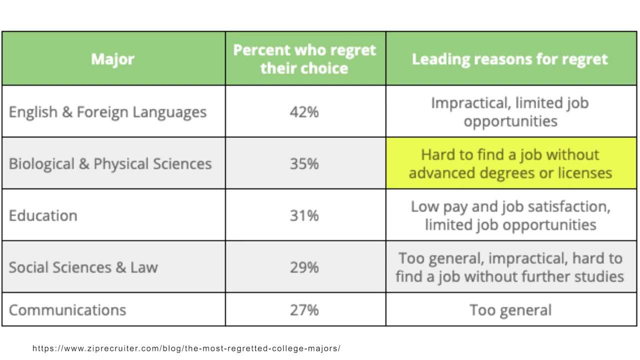 job with just a bachelor's tend to be relatively satisfied with their careers. However, a lot of them are not able to get a job with just a bachelor's, and that's why science-related degrees come in as the second most regretted type of degree, at around 35% of the people. Over one-third of the people who get the degree regret it, But overall this one is above average, and so I'd say that's about average And, like I said before, people who get a science degree, people who love science, tend to really love science, especially the ones that want to work. 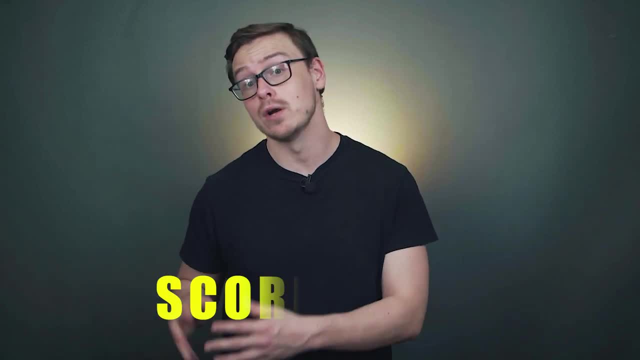 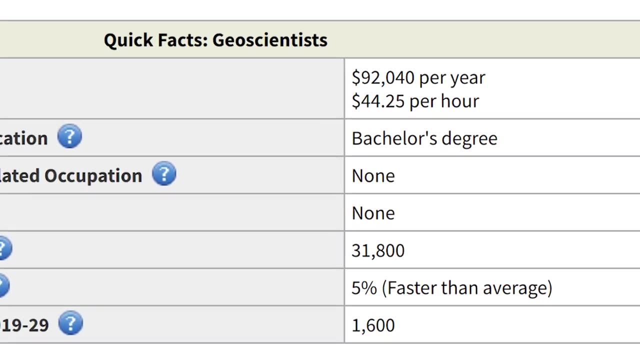 in a career in science, And so I'm going to give this one a score of 8 out of 10.. Next, we're going to be talking about demand, And, going back to the career we were talking about before, which is geoscientists, they are going to be growing at 5%. 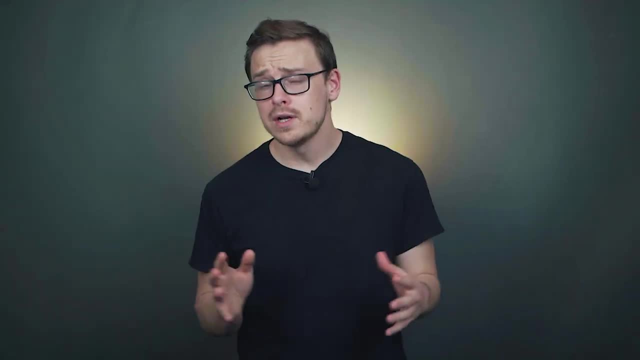 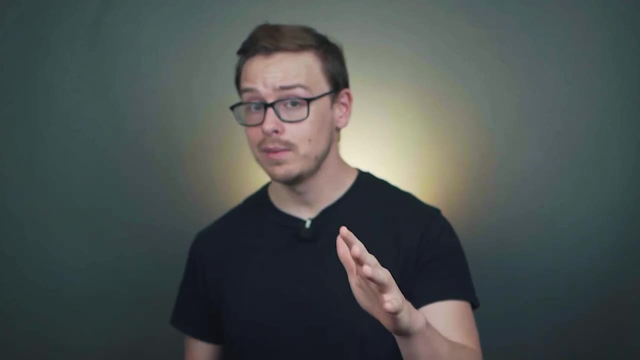 which is faster than average over the next 10 years. Now, one thing I'll say here about geology degrees is: there's a very good chance that you're going to be working in the natural gas industry. Now, the great thing about that is the natural gas industry tends to pay. really well, all across the board, Anywhere from entry-level jobs where you're just getting out of high school and you want to work in labor. A lot of the time you're going to get sent out to the middle of the ocean or, you know, the middle of nowhere where you probably don't want. 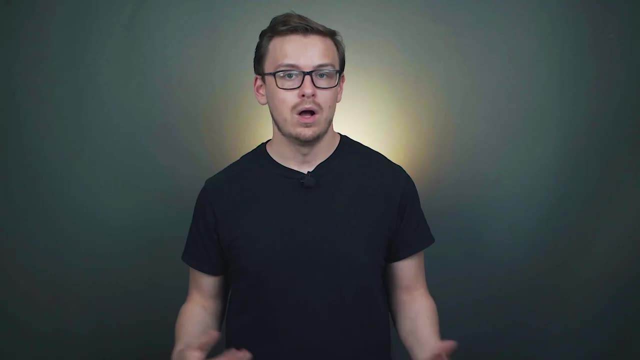 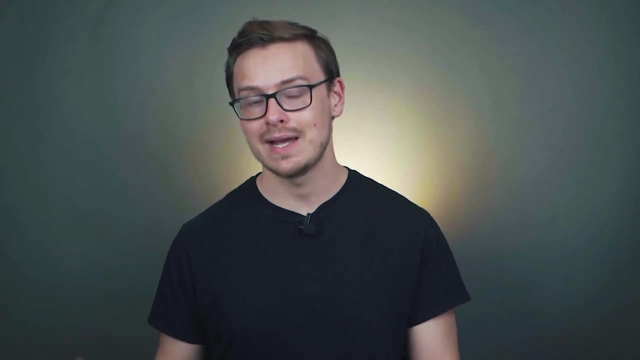 to live, But you can make really good money right off the bat, all the way up to the highest paying degree out there, which is petroleum engineering. Now, unfortunately, the bad part about working in the natural gas industry is that it's very volatile. It's extremely unstable. People are going to get fired when the economy goes down. There could be some kind of tax thing going. we could get into a war, like we did back in the early 2000s, which caused oil prices to go up. All kinds of different weird things can happen which can disrupt the industry. 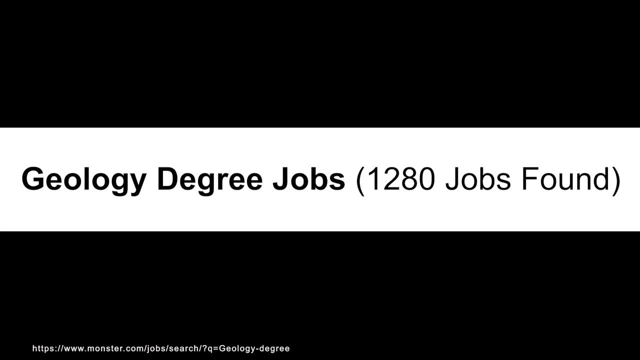 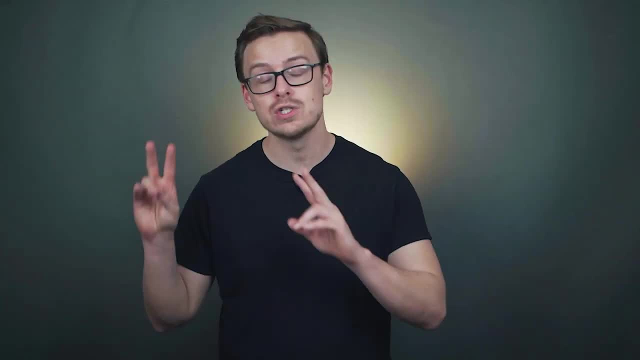 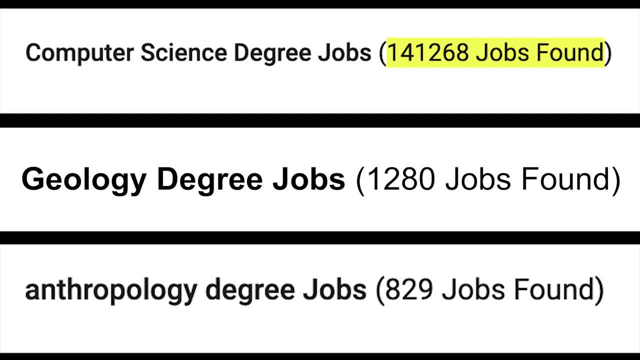 Now when you type in the keyword geology degree onto Monstercom, you'll see that around 1,280 jobs pop up. That means 1,280 job listings had the keyword geology degree somewhere in the post. Compare that to computer science, where over 141,000 did, and then anthropology, where only 829. 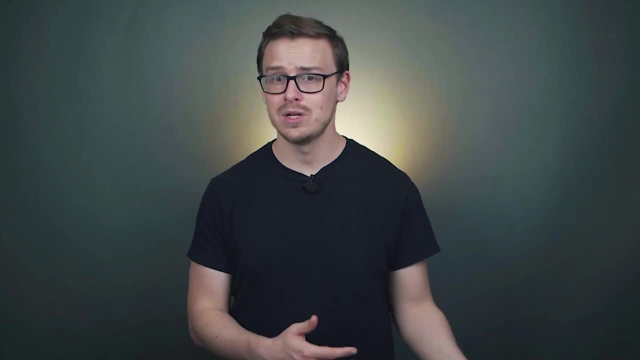 did. So it's a little bit above the average. So it's a little bit above the average. So anthropology, which isn't a great degree, but it's definitely nowhere near something like computer science And that isn't a perfect test by any means. but when you see a really low number, like 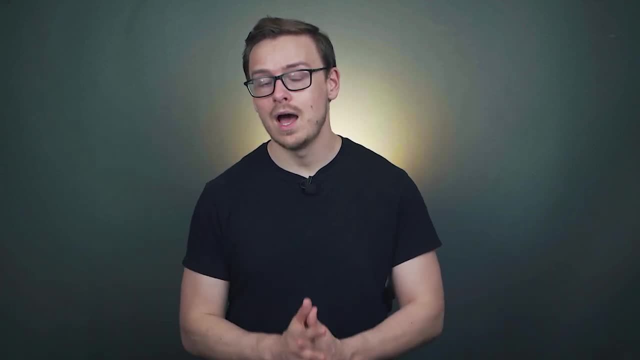 that it can be a little bit of a red flag. So, with all that being said, I'm going to go ahead and give this one a 6.5 out of 10 when it comes to demand. Next, we're going to be talking about 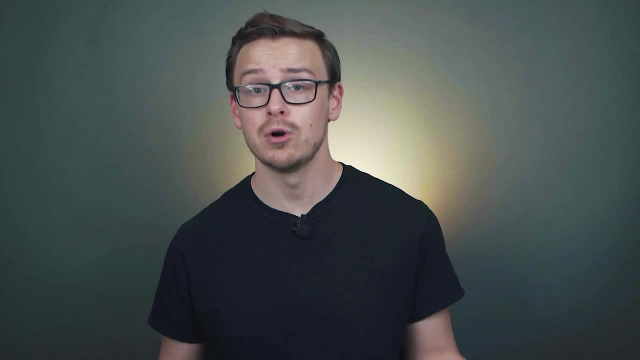 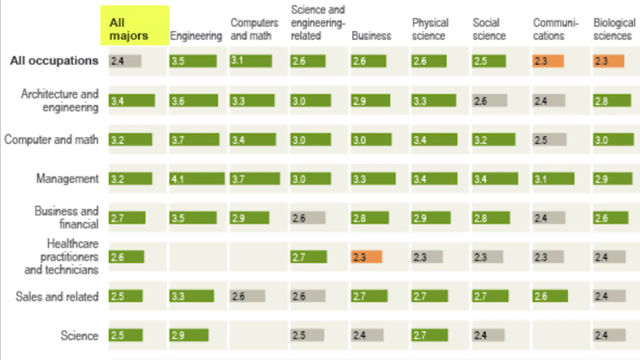 X-factors, and this is going to go over anything that we didn't mention before but I think is still important Now. first of all, when you look at the census data, all college degrees and all different types of careers earn about 2.4%. 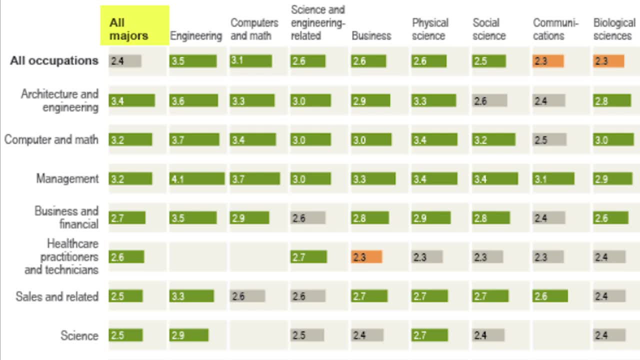 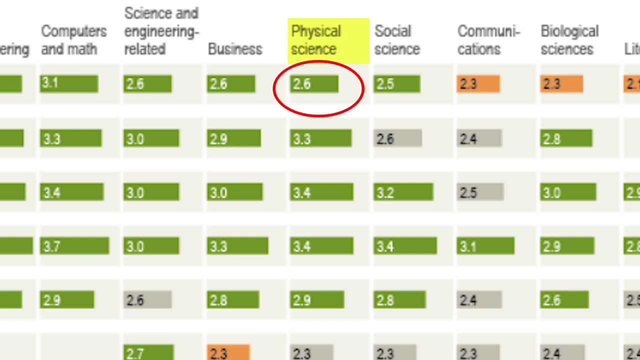 million dollars throughout an entire lifetime. at least they have up to this point. Now, when you look at physical science degrees, which geology is a physical science, it earns around 2.6 million dollars over an entire lifetime. That's going to be a little. 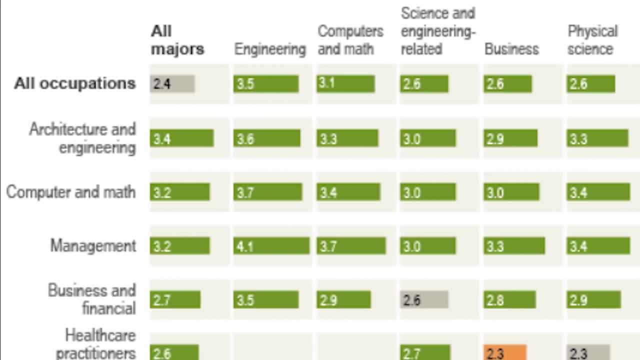 bit above average. so that's a good thing, And you can see when you go down that, depending on what type of career path you go into, you can make a lot more. So, for instance, if you work with computers or you go into management, you'll make a whopping 3.4 million over a lifetime, And 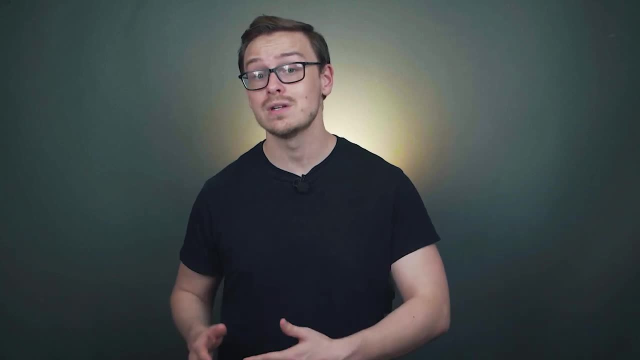 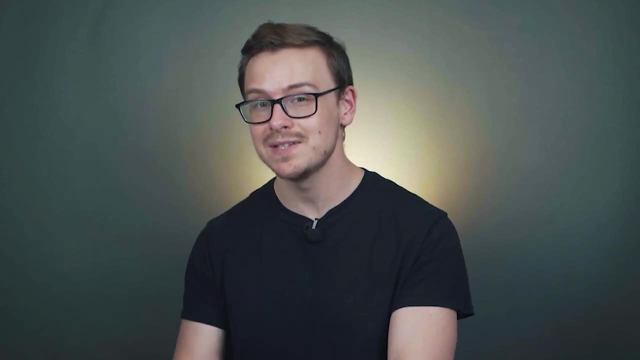 it seems like it's relatively good all the way down the list, and this tells you that it's a somewhat flexible degree. Now, in my opinion, science-related degrees, although they don't necessarily teach you specific skills that you can use in a lot of other jobs and occupations. 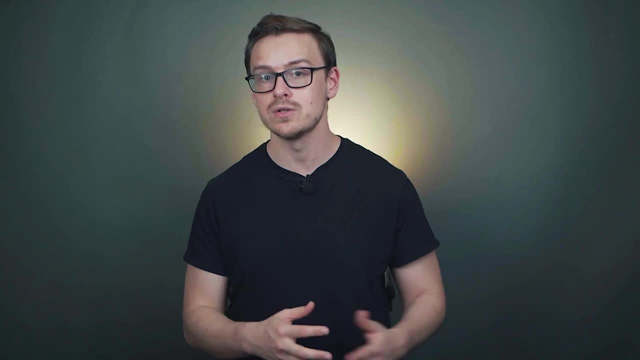 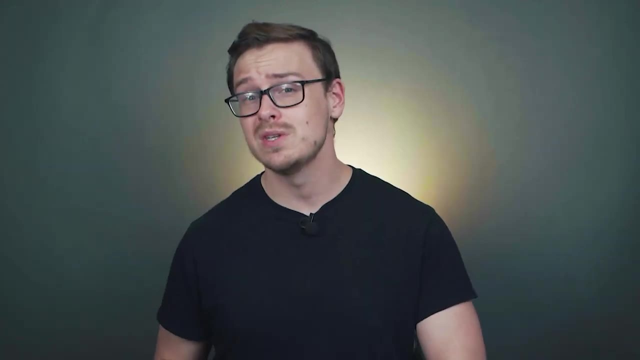 they do teach you what are known as hard skills and soft skills that you can use indirectly in many cases to do really well in other types of careers. Science degrees in general are going to be somewhat respected as well. so let's say you decide you don't want to become a geologist. 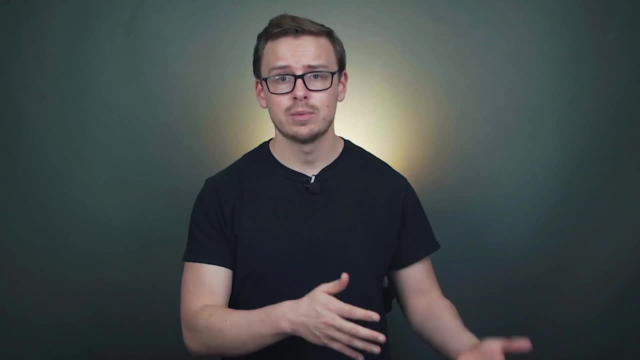 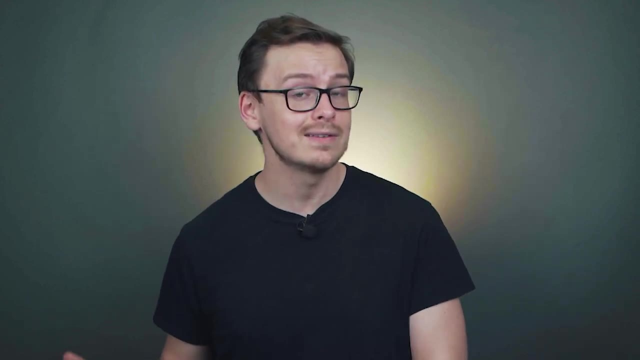 you want to go down a different route. you apply to become a software developer, or maybe you want to work in sales. It tends to be a more respected degree, so people might give you a chance, even though it doesn't necessarily have anything to do with. 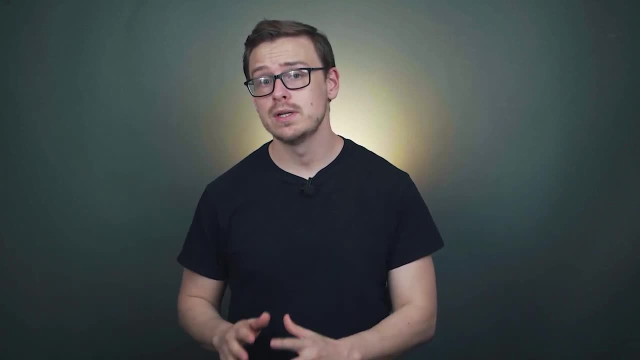 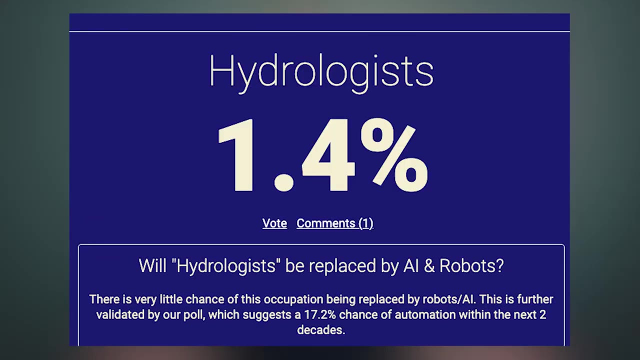 the career you're going for Now. another thing that's great about science-related careers is there's a very low likelihood that they're going to be replaced by robots When it comes to automation and outsourcing. it's very difficult to automate or outsource any type of science-related 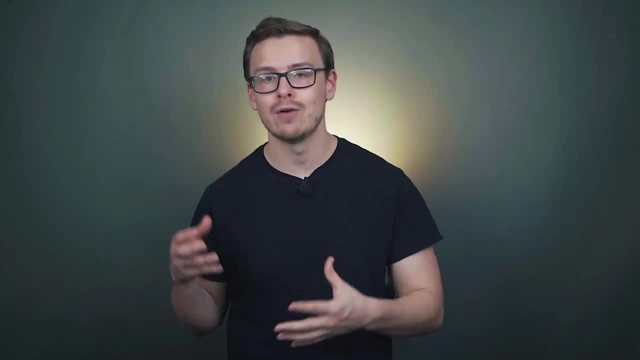 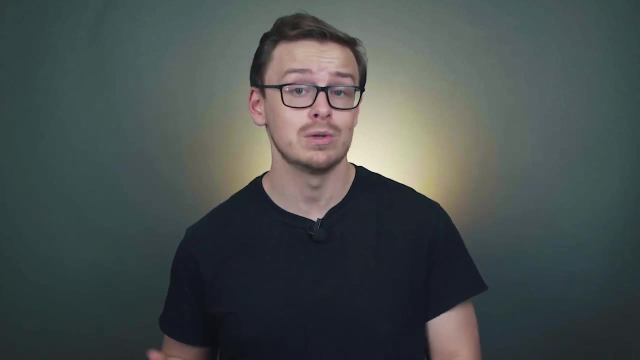 career. You might be able to streamline the processes and have one person do the work of two or something like that, but it's going to be very difficult to completely replace them with robots, so that means that they're going to be relatively future-proof. So, even though geology is relatively 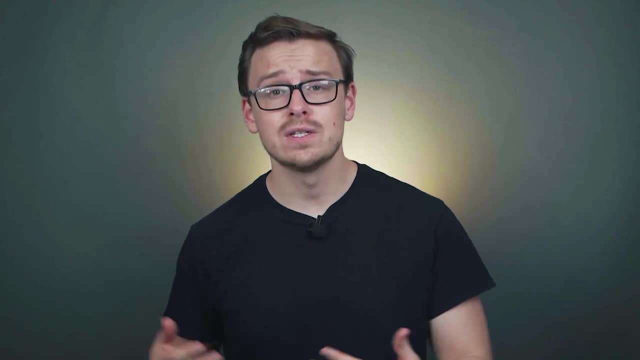 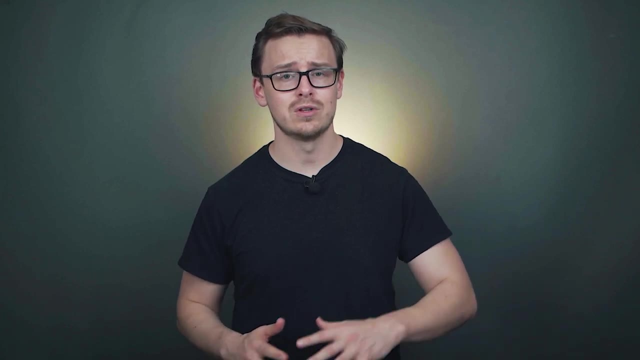 flexible for a science-related degree. there's also a very good chance that you're going to have to move somewhere in order to get your first job, especially if you're going to be working in natural gas. There's a good chance you're going to have to move to the middle of nowhere. 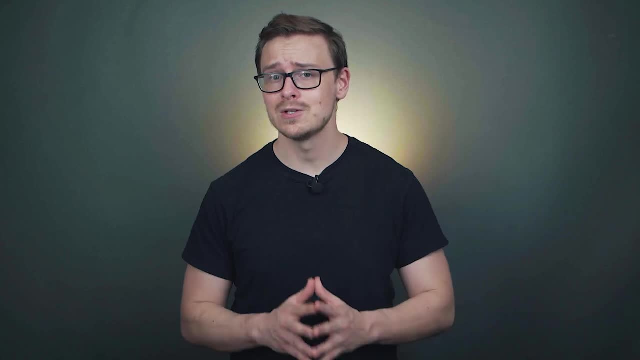 in some oil field or the middle of the ocean for many months at a time, so that's not necessarily good for everyone. If you're someone who has a family and you want to stay close to them, that can be a pretty bad situation. 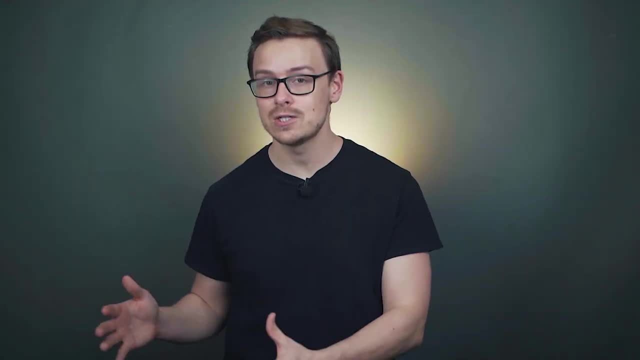 Although a geology degree is going to be relatively flexible for a science degree, compared to all types of degrees like, for instance, compared to a business degree, it's not that flexible. The skill set that you learn is going to be relatively narrow, compared to an engineering degree, for instance, where the skills you learn can be applied to just 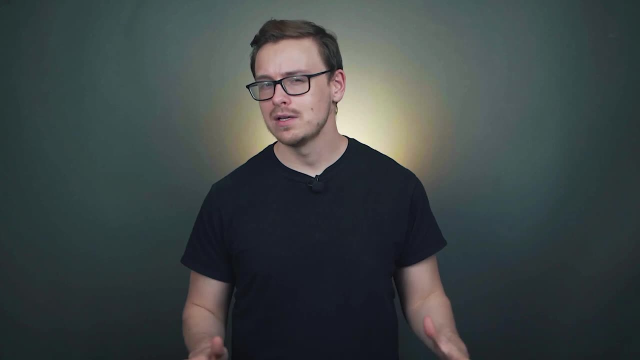 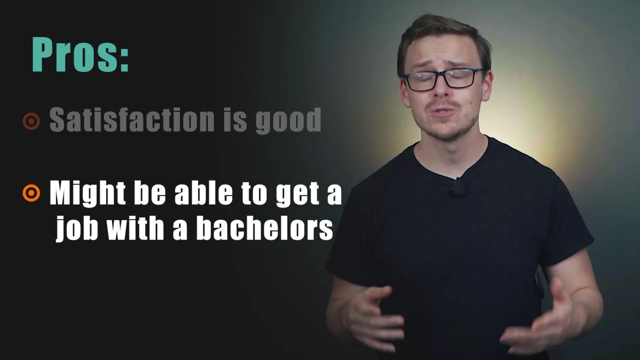 about anything out there. So overall, when it comes to x-factors, I'm going to give this one a score of 7 out of 10.. So the pros here are going to be that the satisfaction is relatively good. You might be able to actually get a job with a four-year degree, which is great. 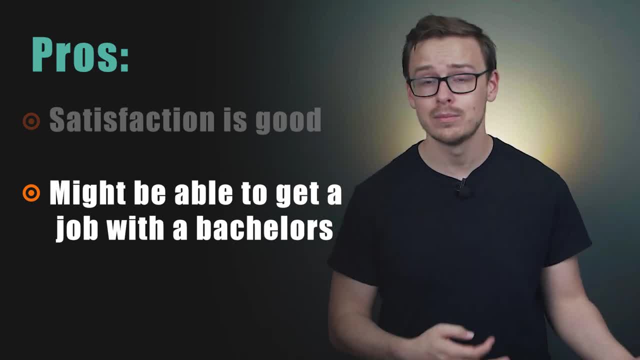 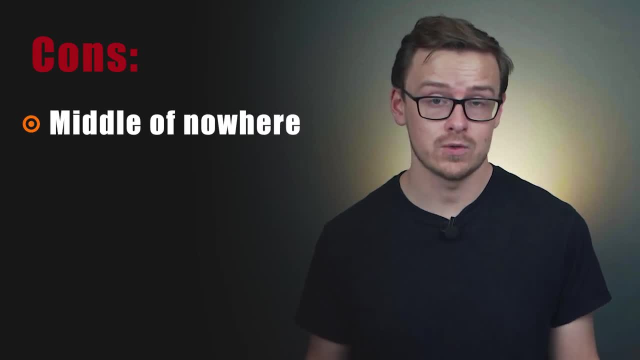 compared to all the other science degrees- or not all of them, but a lot of them- And the salary is going to be fairly good, especially if you want to work in the natural gas industry. Cons here are that if you do work in the natural gas industry, you're going to be 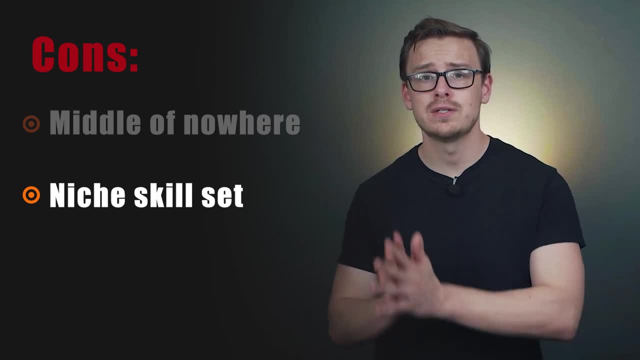 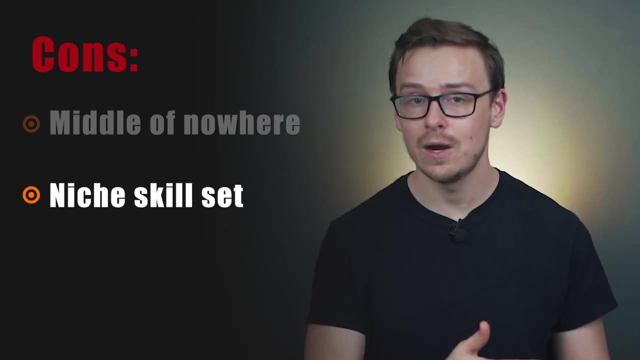 in the middle of nowhere. The skill set that you learn is going to be relatively niche. You're going to learn skills that are very specific to geology, and some of those skills might indirectly carry over to other careers, but probably not directly. 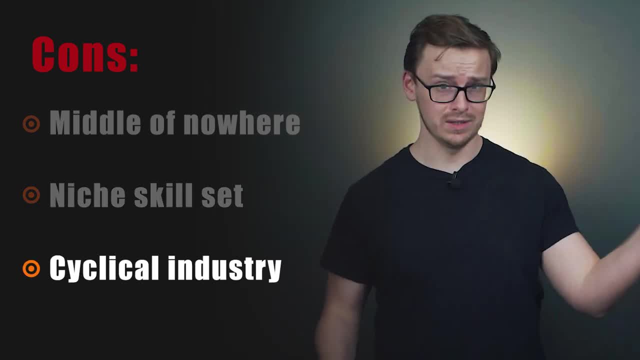 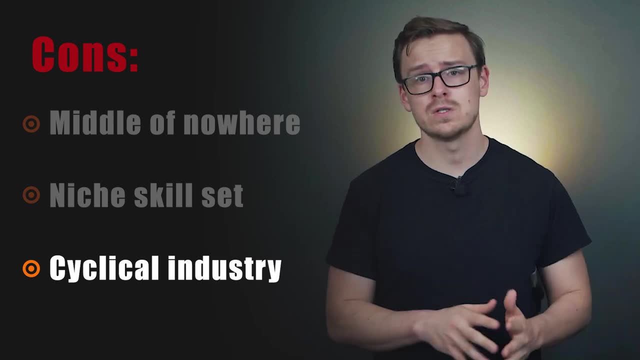 And then natural gas is a very cyclical industry, so it might be really good for five or ten years and then really bad the next five or ten years, And who knows what's going to happen with electric cars and nuclear energy and all kinds of other stuff going on right now. So overall, 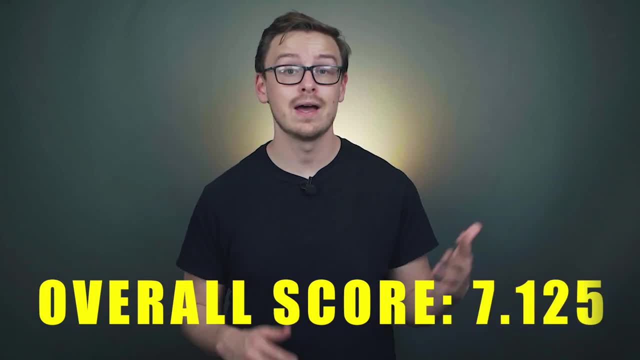 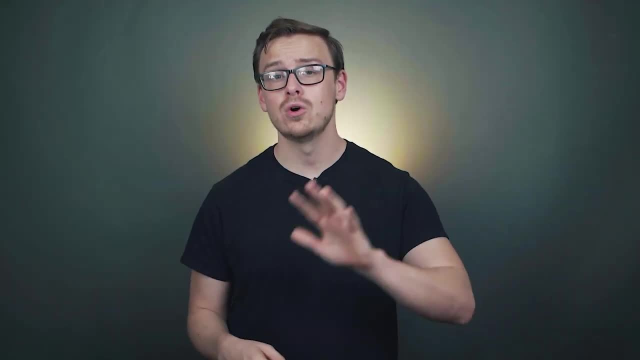 I'm going to give this one a score of 7.125 out of 10.. So that's pretty good, as long as you do your research and you know exactly what you're getting yourself into. You have a plan, you know what careers you're going for, and then you talk to people who are 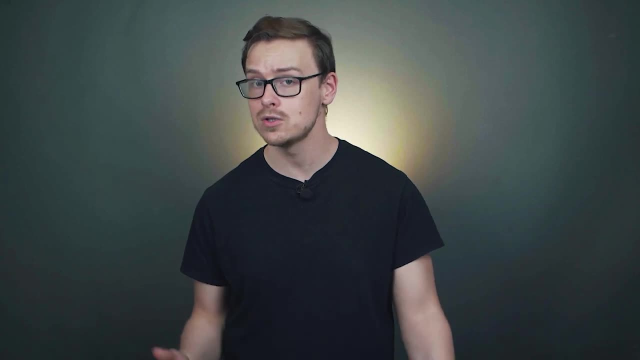 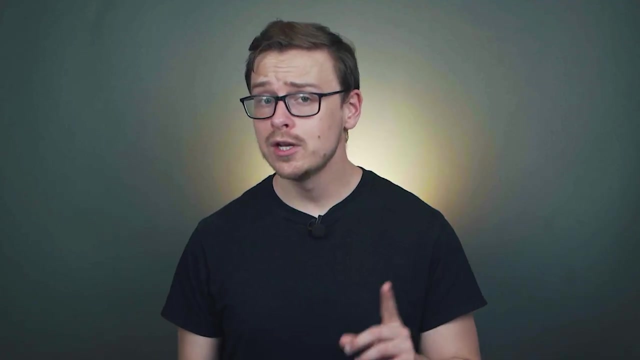 in those careers. You're networking, you're learning skills, you're doing internships. I think if you do all those things the correct way, which I talk about in a lot of my videos, you should be okay. Now, if you do end up having to go to graduate school- the good thing about 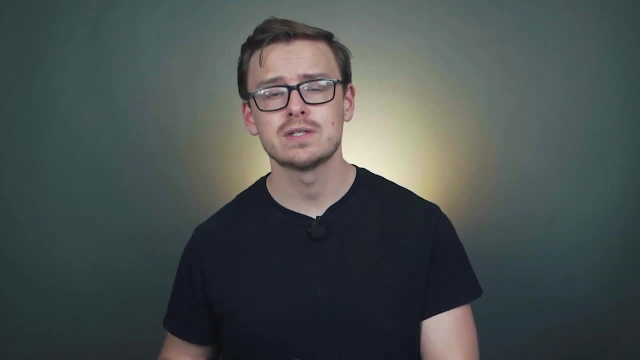 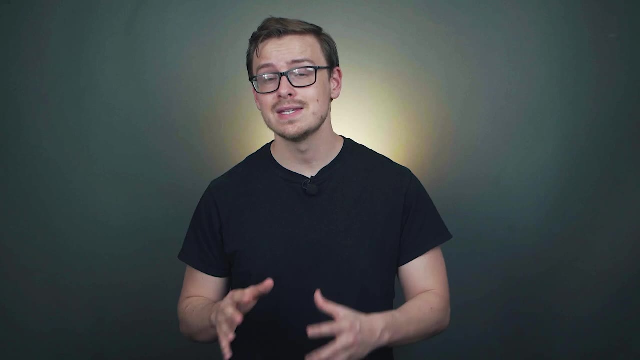 some of the science-related degrees is there's a good chance that you'll get some kind of fellowship or scholarship that'll pay for a lot of it. There's still going to be a lot of time commitment, of course, but the good thing is this type of PhD, a lot of types of PhDs out there- you have to pay. 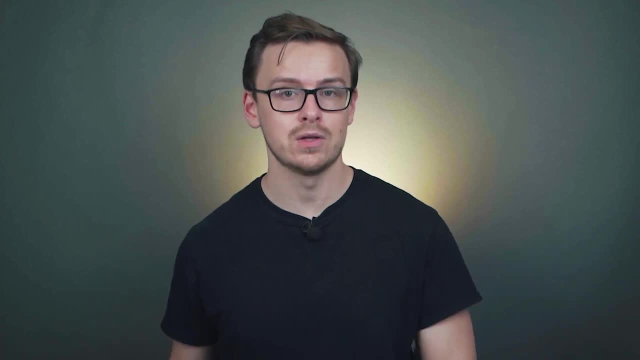 for, but this particular one, there's a good chance that you can find a fellowship. It might also be a good idea for you to take extra classes, learn extra skills, maybe minor or double major, and something that would make your degree look a little better. 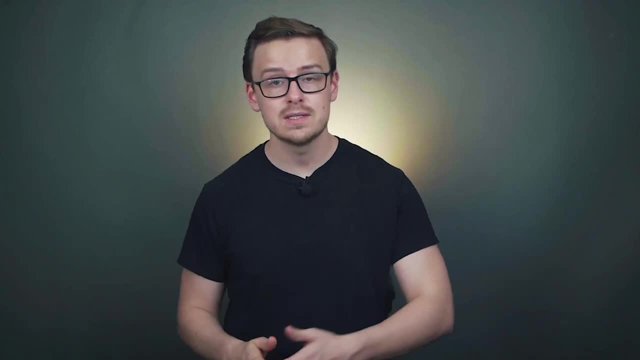 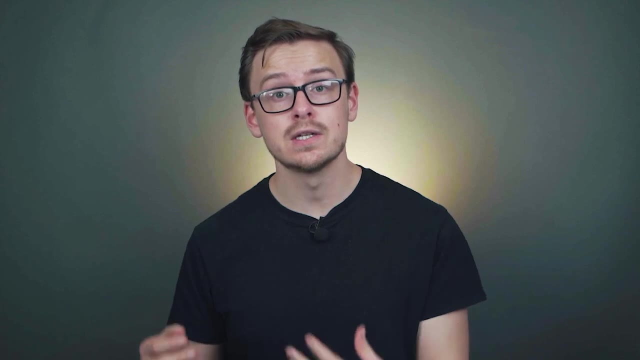 Better to a potential employer. Learning technology-related skills, mathematics, statistics- all of these sorts of things are going to help you out, As, with a lot of careers out there, the toughest thing is to get your very first job out of college. 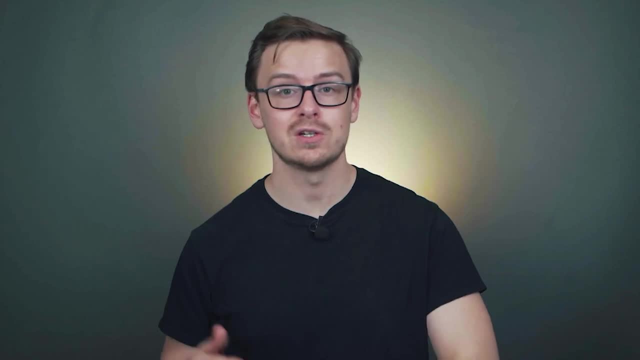 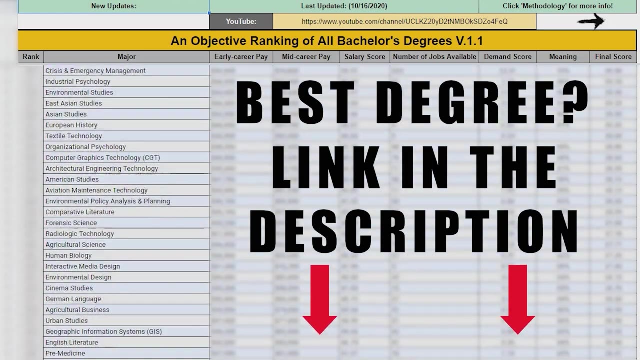 Once you get two or three years of experience, it's going to be much easier for you to get your second and third job etc. And to help you with your research. if you want to check out my Patreon down below, I have the college degree ranker version 1.1 at this point, but maybe by the time